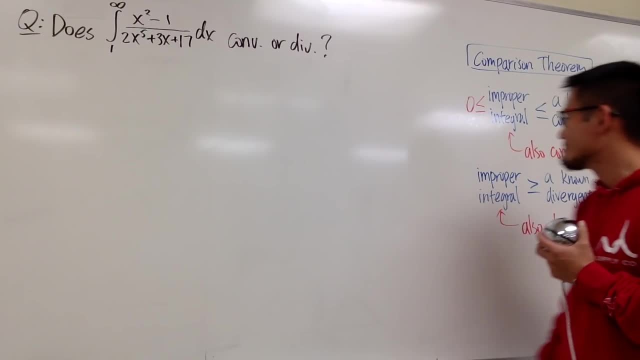 Just always do it like this way. It's more consistent. alright, If you can show that, the improper integral that you're trying to work out. if this is less than or equal to something that you know already to be convergent, well, once again, convergent means that you have a finite value. 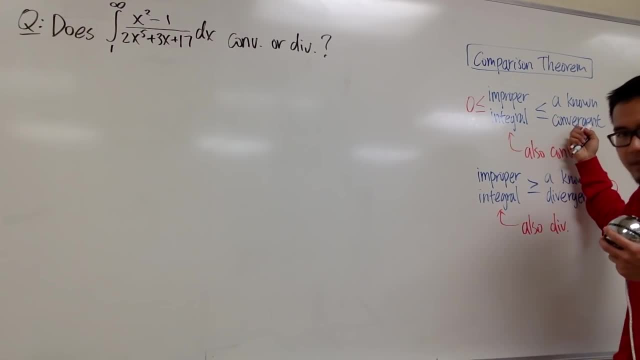 What you're showing is that something is less than or equal to a finite value. Okay, Of course, you can draw a conclusion that this right here has to be finite as well, isn't it? So, in other words, this improper integral has to also converge. 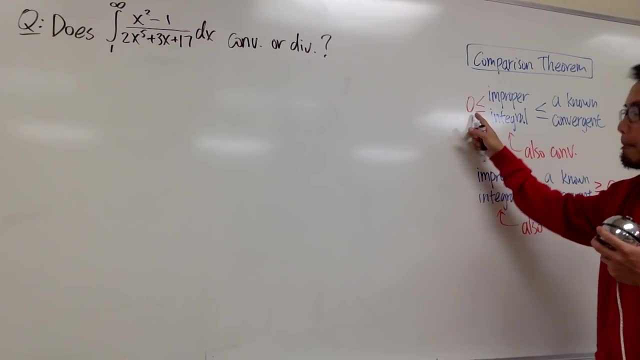 And here's a small detail, though: We want both of these to be positive right, Because I don't want to say, alright, negative infinity is less than or equal to positive 2. I don't want negative infinity to be right here. 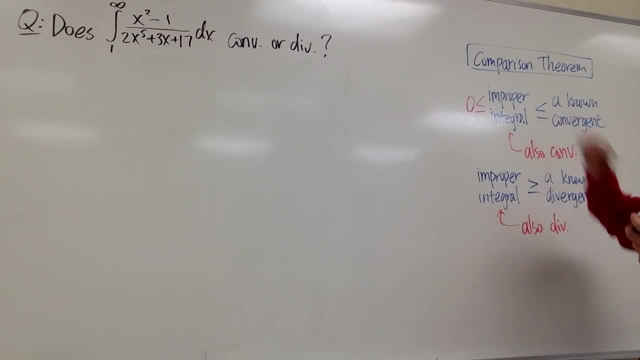 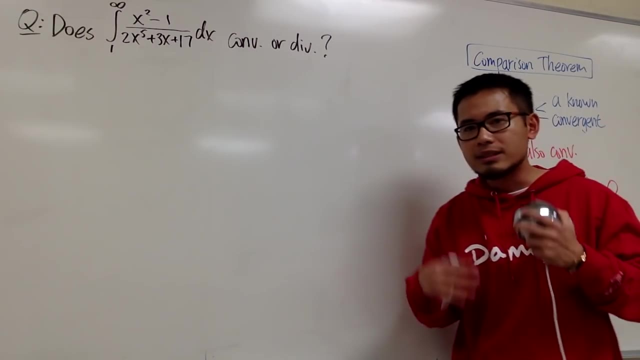 So all the problems that will work out right now, it will be just all positive And I will point out the details. And I will point out the details along the way. But here is the first idea And of course sometimes you may come up with something and that happens to be diverges right. 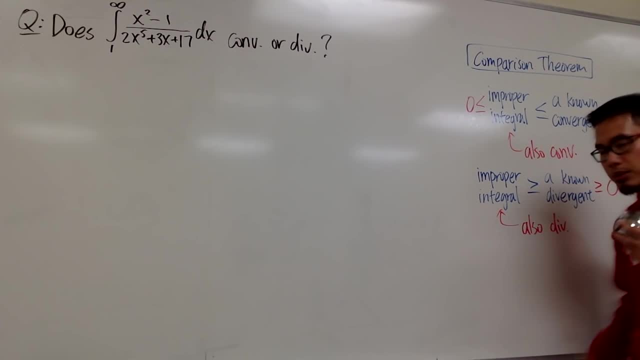 Right here if you have a non-divergent. in this case, remember, a divergent means infinity And if you want to make this all positive, this right here, representing positive infinity, If you can show, the improper integral that you're trying to work out is greater than or equal to a divergent. 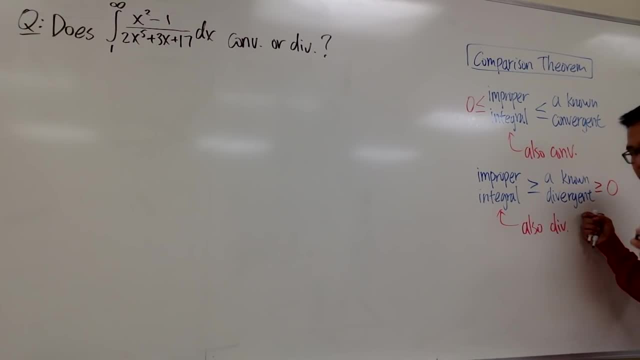 greater than or equal to infinity. That means you can draw a conclusion that this has to be even a bigger infinity. right, So you can say this right here also diverges, and once again, both of them have to be greater than zero. 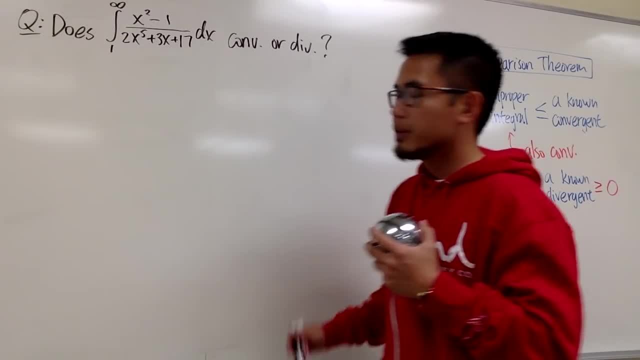 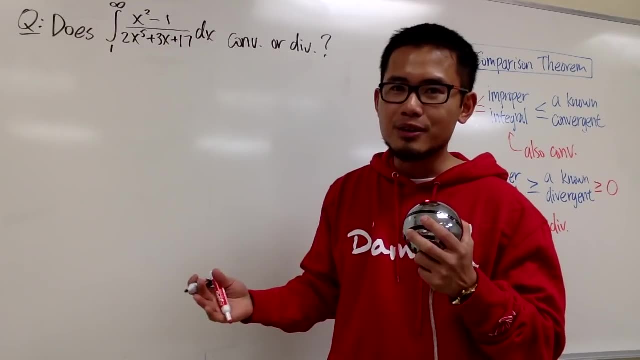 That's the detail and that's the idea. So here is the work Right here. this is what we have. I want to first come with something that I know much better and I can draw a conclusion right away And whenever we have a rational function inside, this is how we can do it. 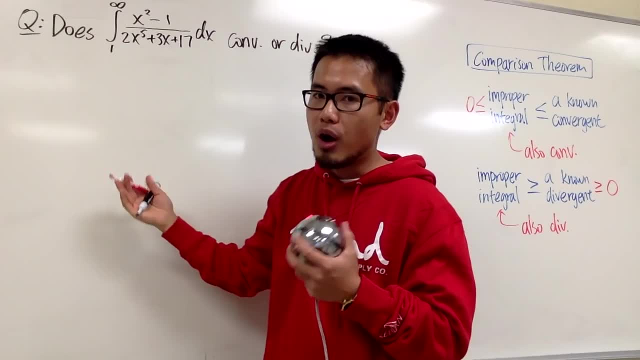 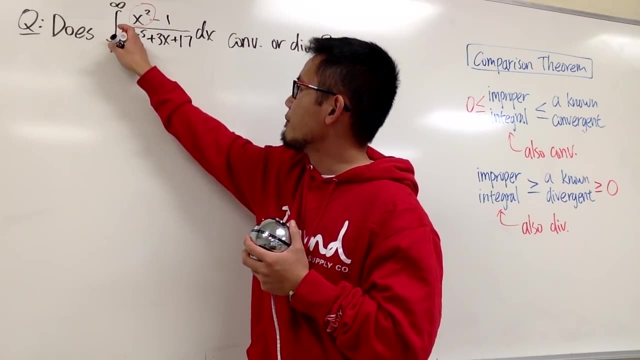 On the top. let's just go ahead and pick the dominating part, namely the highest power of x, which is the x squared, And we do the same on the bottom. In this case, we have 2x to the 5th power. 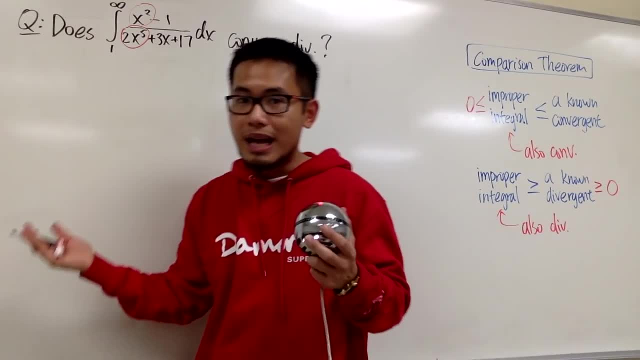 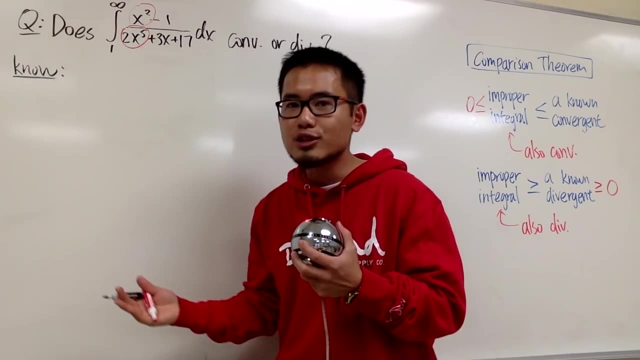 Like that, right, And I think we know that part much better. and let me just put it down: Always put down what you know first. It's just like an introduction when you're trying to write an essay, right? Anyways, we will put this down as 1.. 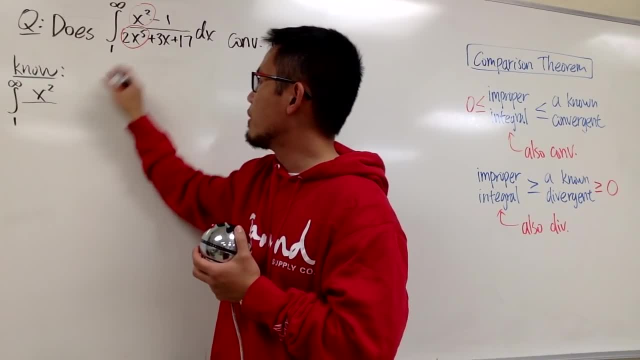 1 to infinity On the top. I will just write down x squared Over on the bottom. I just care about 2x to the 5th power Like this, And of course we can simplify the powers. 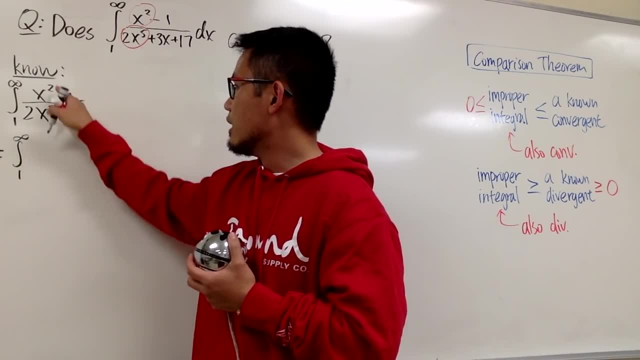 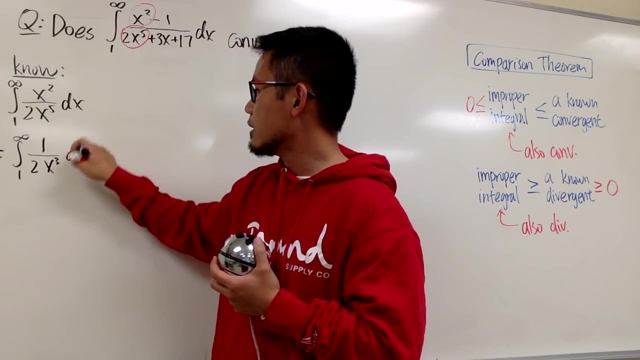 This is going to be integral from 1 to infinity. On the top, just 1.. On the bottom, I have 2. And we have x to the 3rd power, now The x right, And we have 1 over 2.. 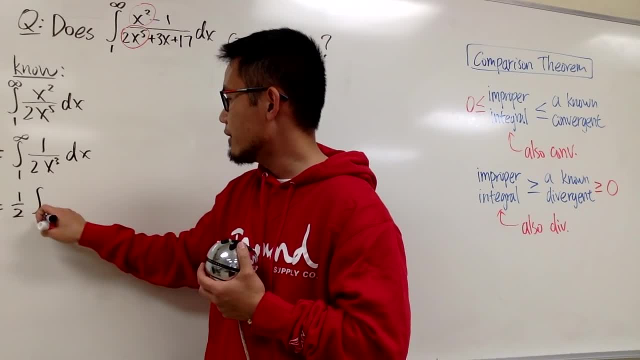 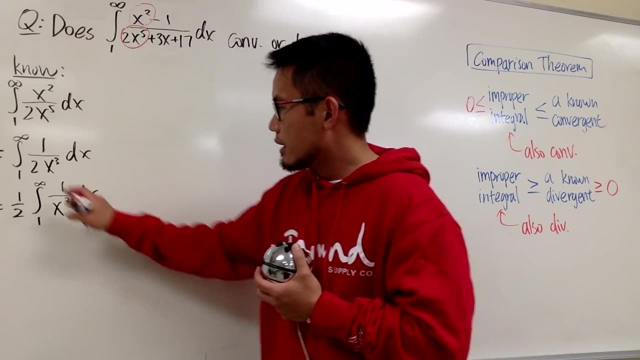 We can take that constant multiple out: 1 half integral, 1 to infinity, 1 over 2.. 1 over x to the 3rd power, dx. Okay, This part right here. we have a theorem for that. 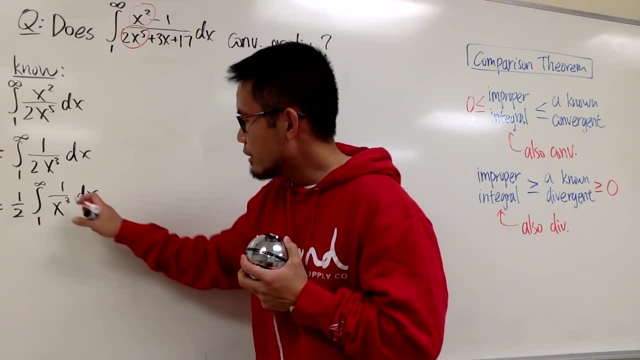 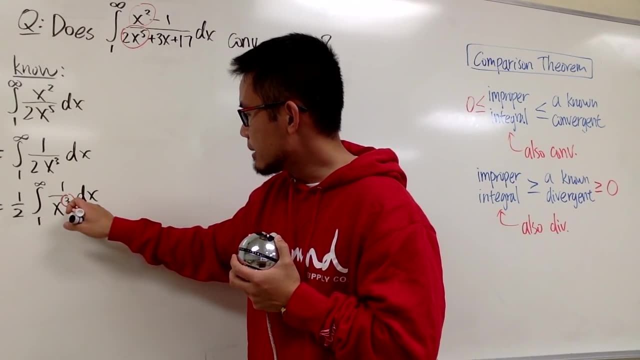 That's the p-test, or the p-integral right, And you see that that's the version 1, because we have infinite interval from 1 to infinity Right here. this is the power p. p in this case is equal to 3.. 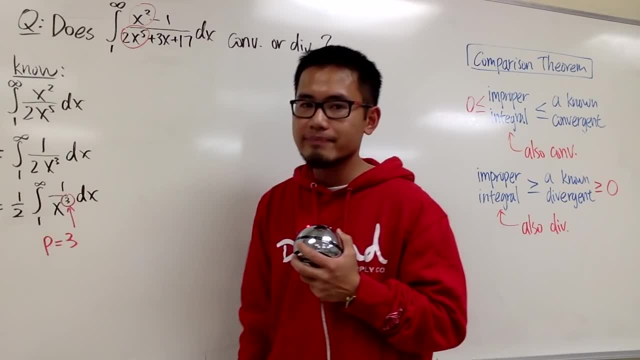 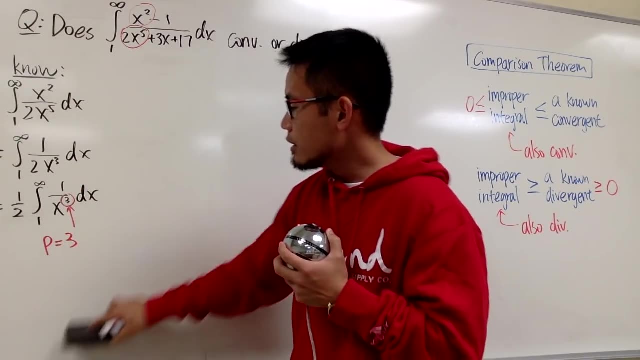 And for type 1 situation, when we are going from 1 to infinity, if p is greater than 1, we know this right here, converges, Okay, So in this case don't just write down: p is equal to 3.. 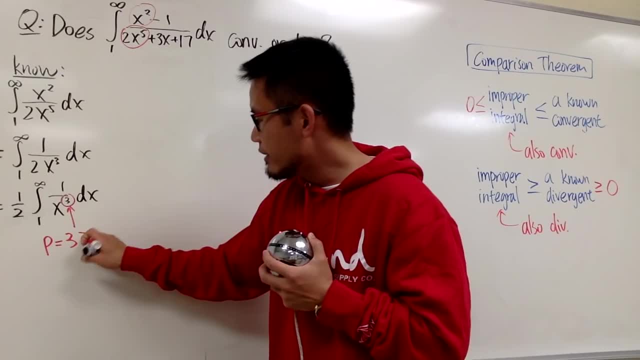 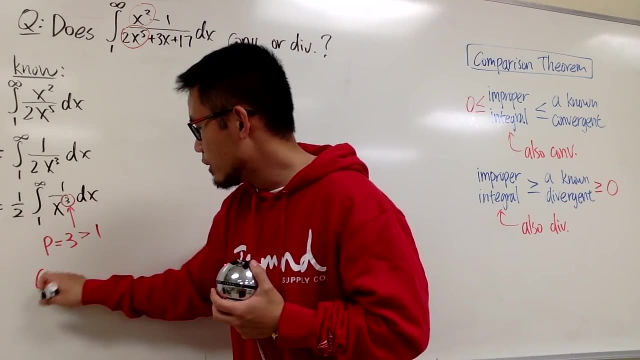 You have to indicate that 3 is greater than 1, because you are trying to say p is greater than 1.. In another word, you can finally say that this is a convergent, This is finite And, of course, if you are just multiplying by 1, half, 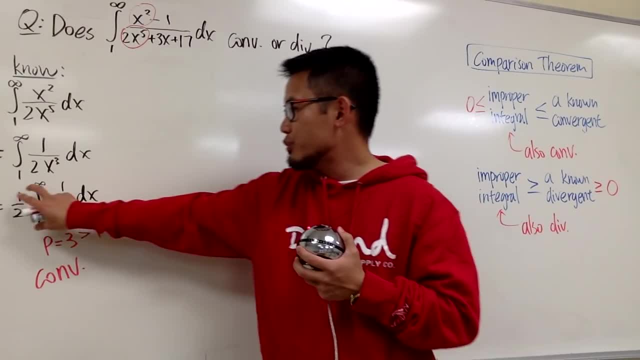 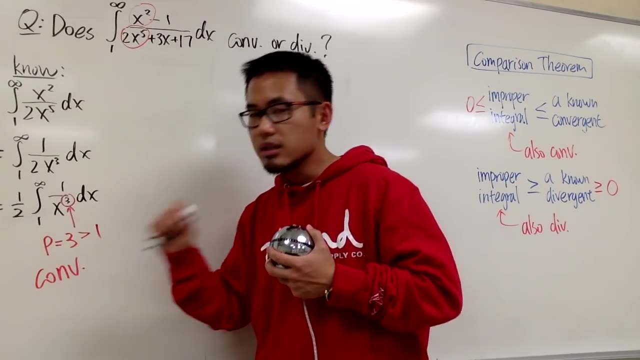 it is still finite, So you don't really need to worry about the 1 half. if you don't want to, Right, But that's all we care about is the integral part. It's convergent, Okay, Now, that's what we know. 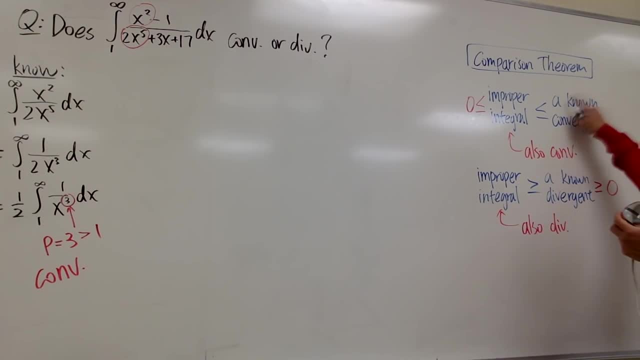 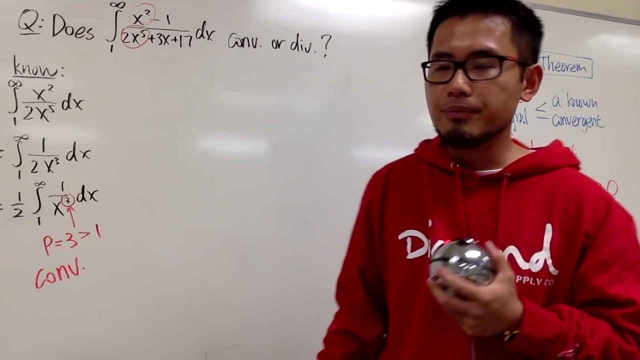 And we are looking for this first situation because I have something that I know to be convergent first right. So I'm trying to set up this inequality the less than situation and hopefully I can build up that inequality and I can show you guys that that inequality is true. 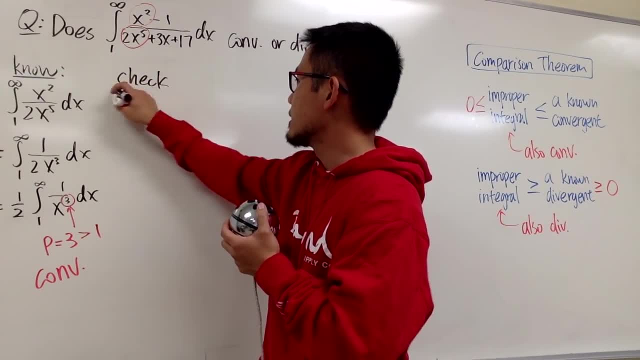 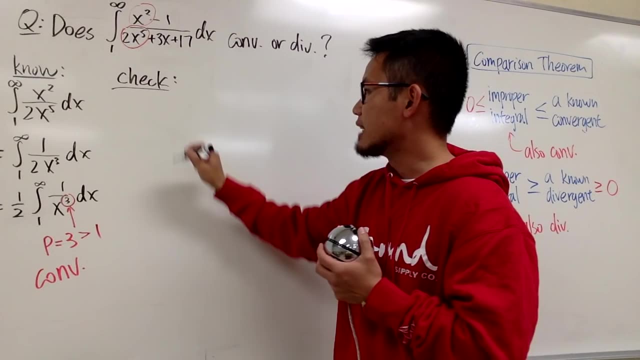 And now we will have to do the following check. The following check is that I will put down the improper integral that we are trying to find out right here on the left-hand side. So I will write down this integral from 1 to infinity. 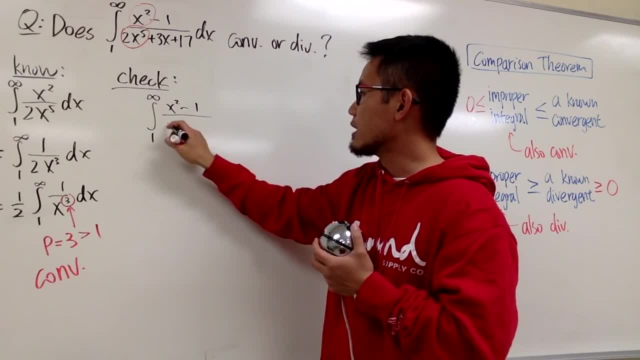 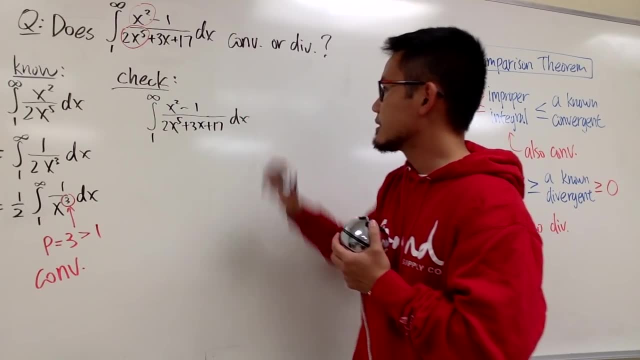 On the top is x squared minus 1, over on the bottom is 2x to the 5, plus 3x and then plus 17 dx, And I will put down the things that we know much better on the right-hand side. 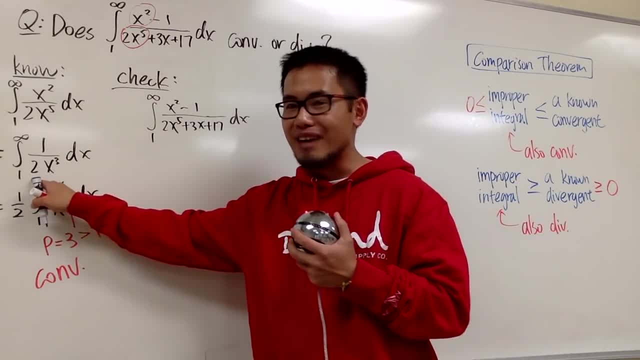 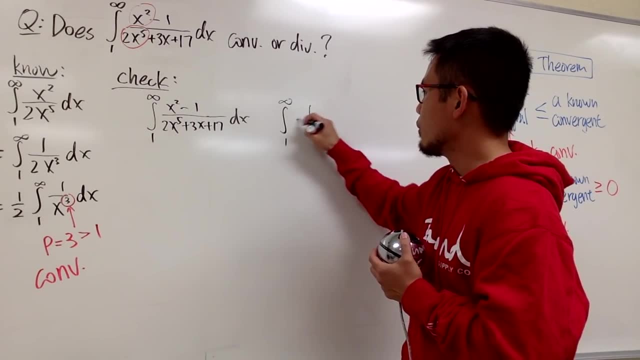 Don't put this down. Put this down better, because we need to have that one-half right here. And you'll see, right here I'll put down integral from 1 to infinity, 1 over 2x to the 3rd power, dx. 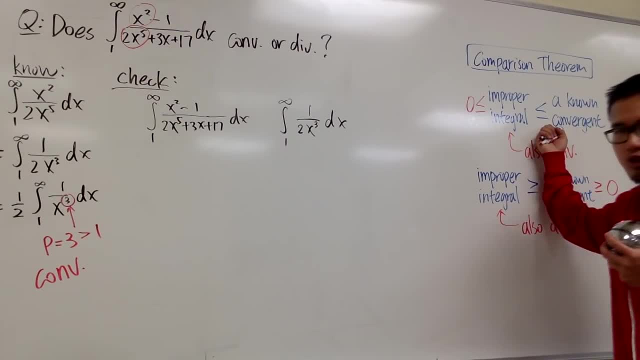 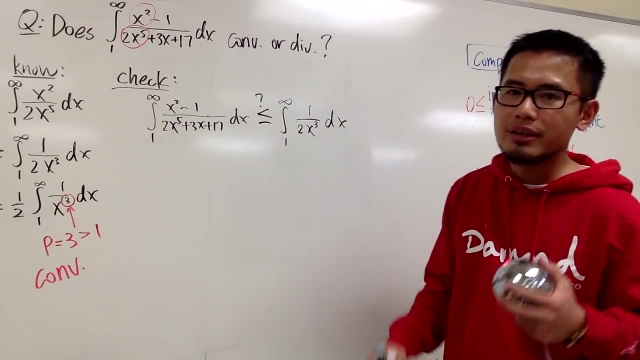 Okay, And in between I need to show you guys and convince you guys. this is less than or equal to, But in fact I don't know yet. So technically I have to put down a question mark. Okay, All right. 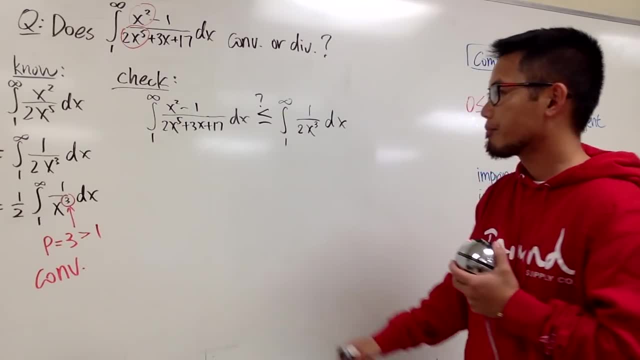 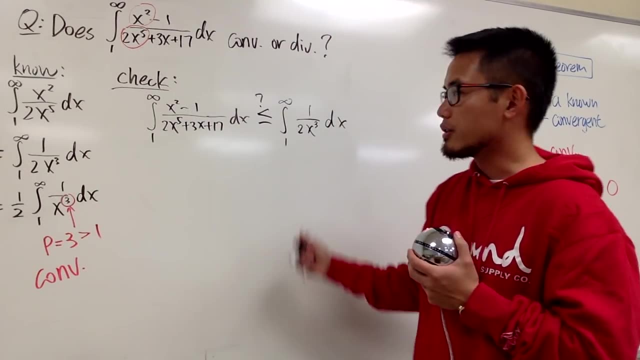 So this is what we have at the moment, And now you see both integrals. they are going from 1 to infinity. I just have to compare the inside. So in other words, I'm just looking at this as x squared minus 1, over 2x to the 5th power. 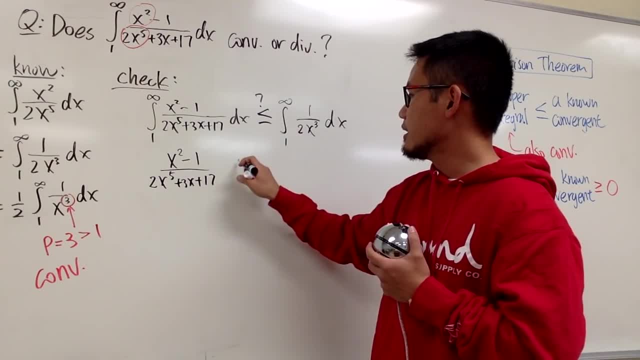 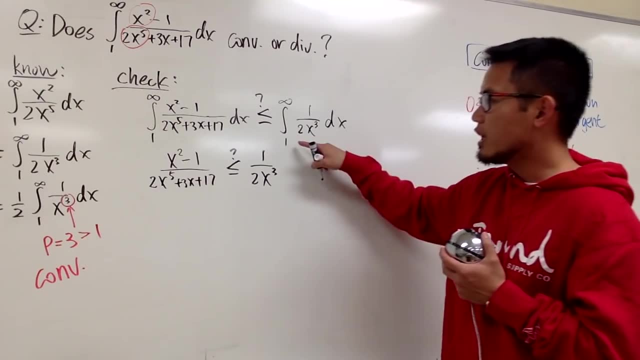 plus 3x plus 17.. And then is this less than or equal to 1 over 2x to the 3rd power, And right here we only care about the x values going from 1 to infinity. So I will say that: 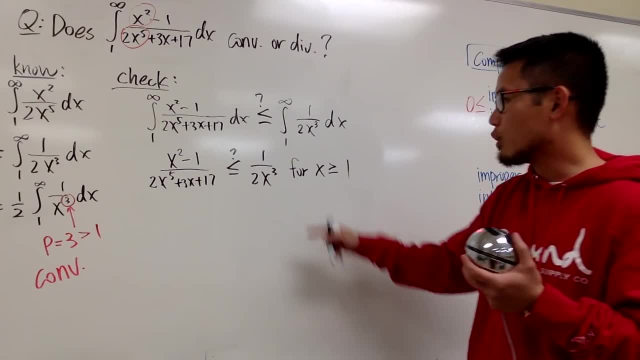 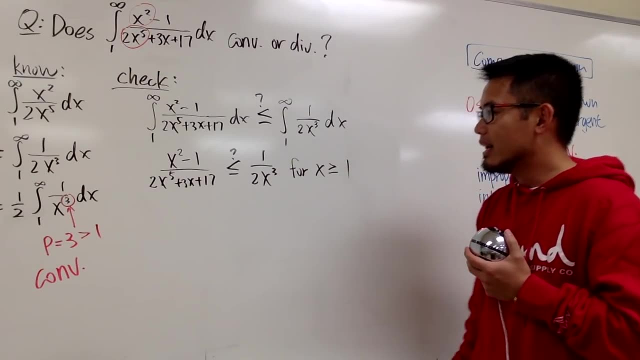 4x is greater than or equal to 1, and, of course, if you are talking about 5 to infinity, right here you put down: 4x is greater than or equal to 5.. And the deal is that, right here, 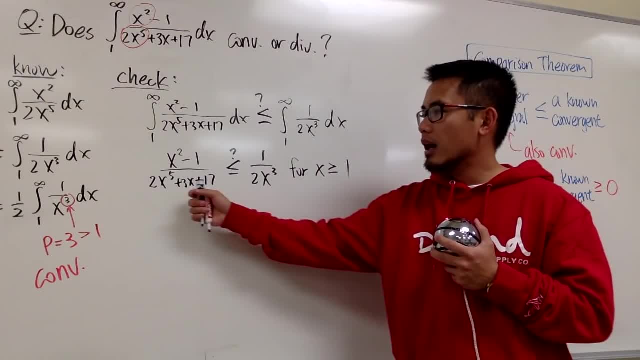 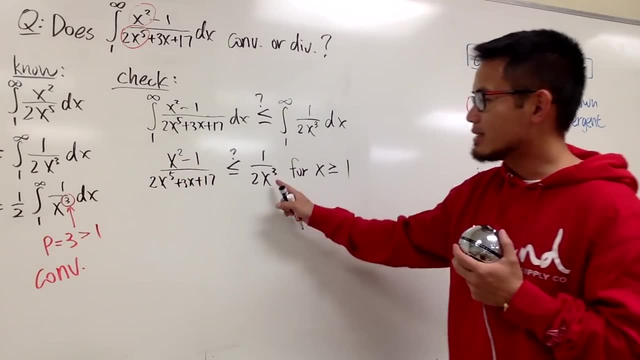 or maybe right here, when x is greater than or equal to 1,. on the left-hand side, the smallest you can get is 0, but it's okay. But then you will always be positive afterward. Likewise on the right-hand side. 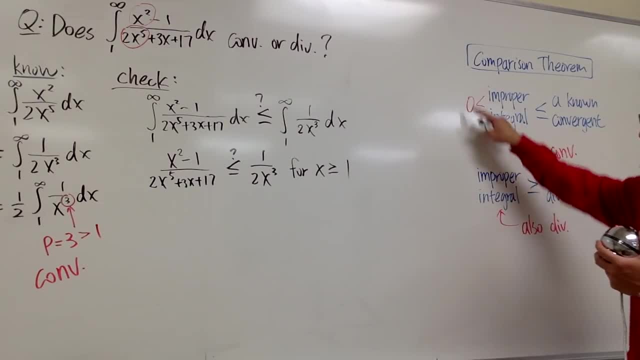 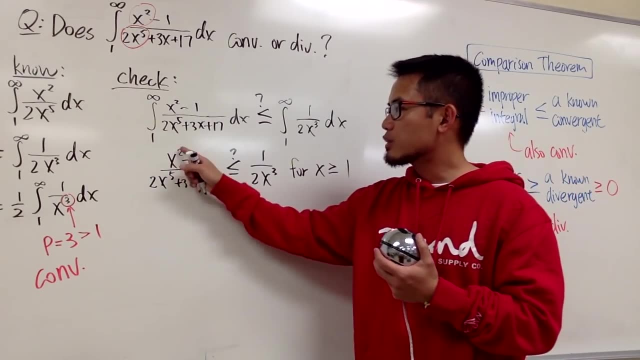 it's always going to be positive as well. So that's this part. Okay, that's this part right here. Now the deal is that if x is greater than or equal to 1, x squared minus 1, it will be positive. 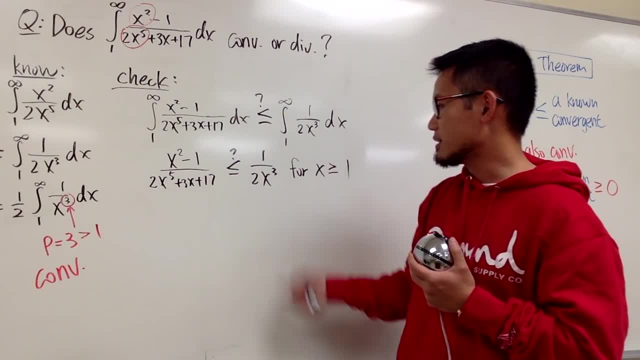 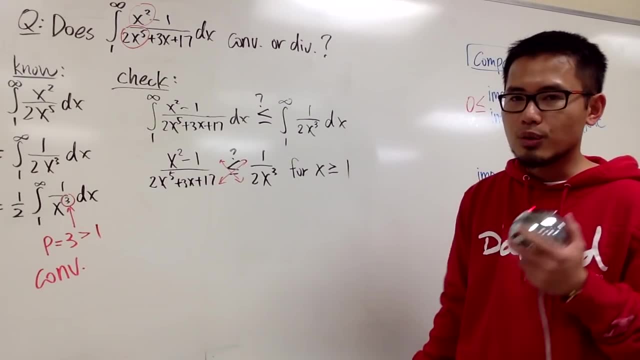 On the bottom. it's always positive. 1 is just positive. This is always going to be positive as well. So that means I can just cross-multiply. Right, I can just cross-multiply, In fact, if you would like. 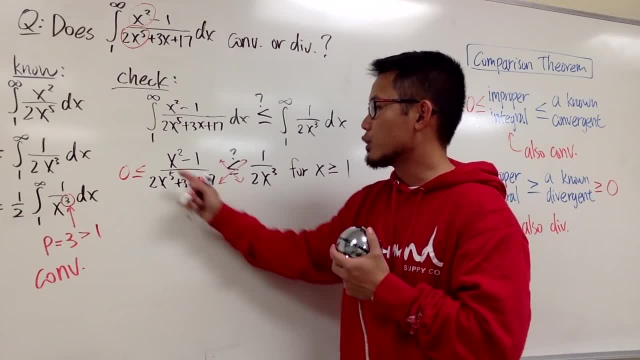 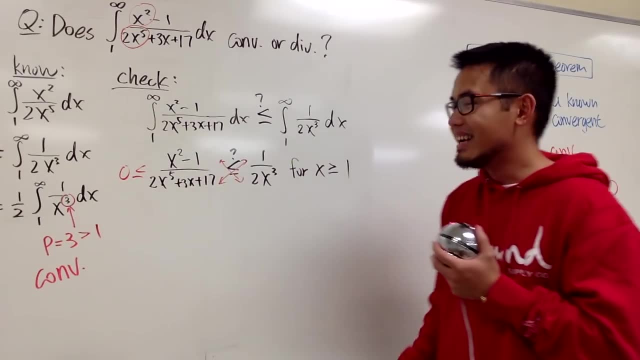 I can just indicate that it's always. both of them are always greater than or equal to 0. When x is equal to 1, it is exactly 0, but it's okay, right, You have the equal sign, Anyways. 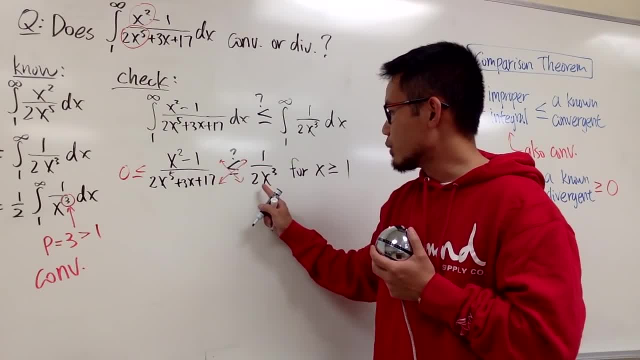 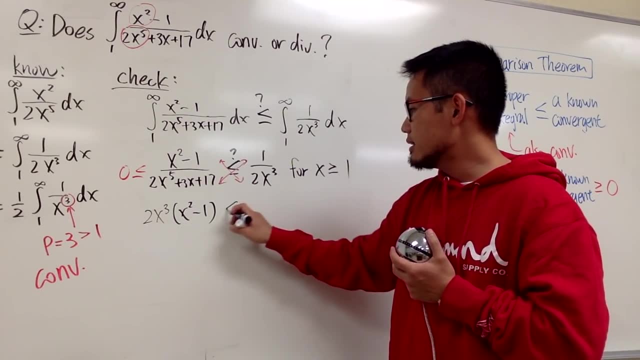 I will just cross-multiply right here. So let me just show you guys the work: 2x cubed times that right. So put down 2x cubed times that x squared minus 1.. And then is this less than or equal to: 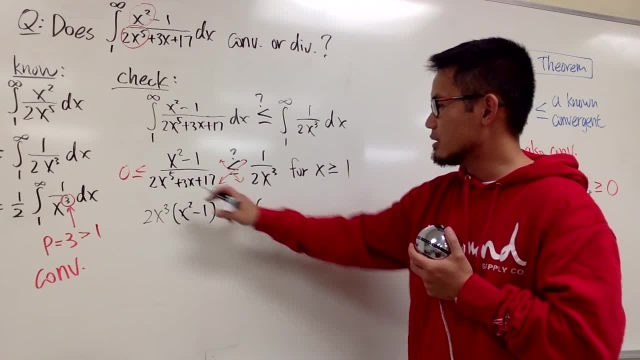 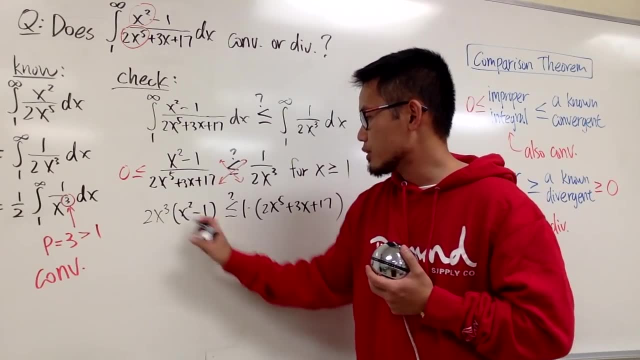 that times 1, which you put down, 1 times this: 2x to the 5th power, plus 3x plus 17.. And now, of course, distribute, So we have 2x to the 5th power. 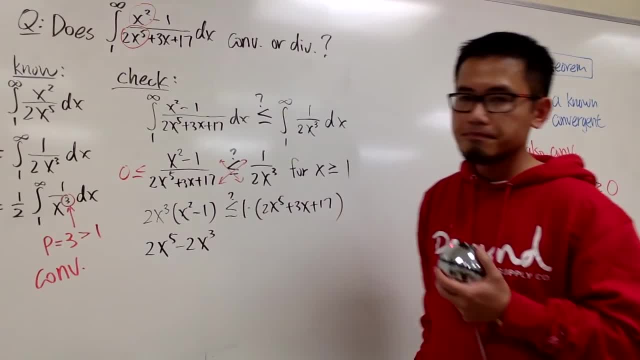 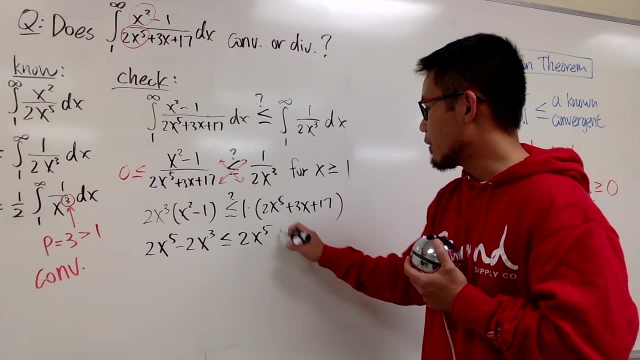 This times, that is minus 2x to the 3rd power, And here we will have less than or equal to 1 times. this is just 2x to the 5th power plus 3x minus plus 17.. Like that right? 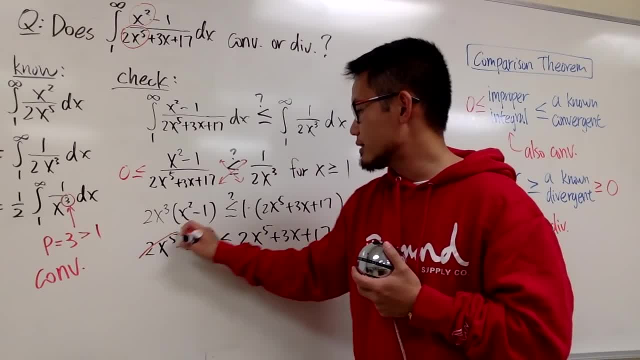 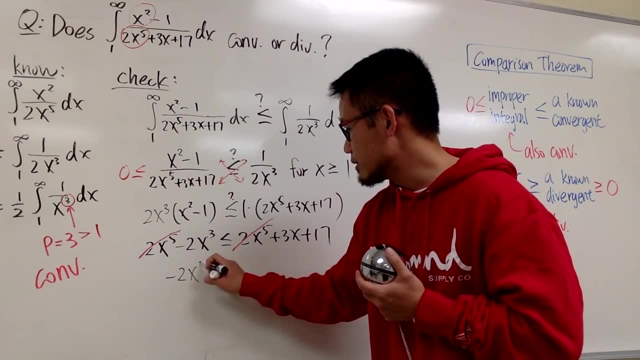 Okay, is this true or false? Well, if you would like, I can just cancel this out. Right And on the left-hand side, you have nothing but just negative 2x to the 3rd power, And this is less than or equal to that. 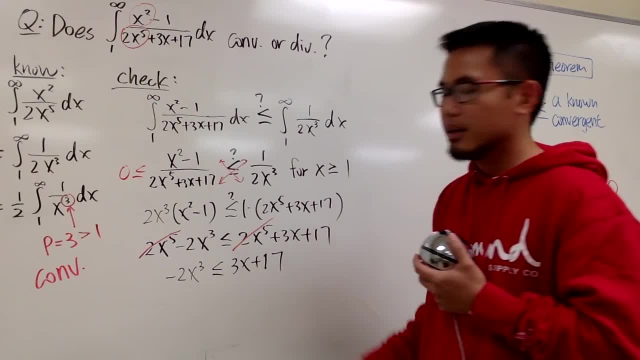 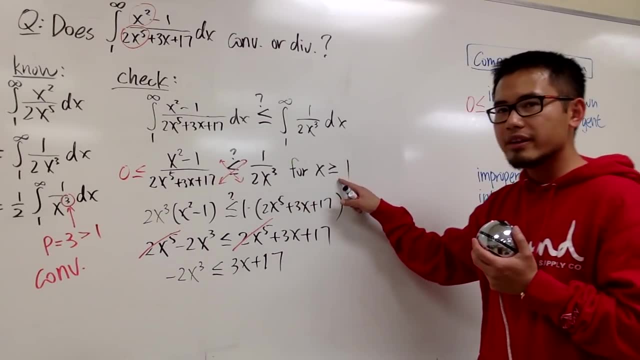 3x plus 17.. Is this true or false? This right here, is true because x is greater than or equal to 1.. You can imagine if you plug in 1 right here on the left-hand side, you have negative 2. 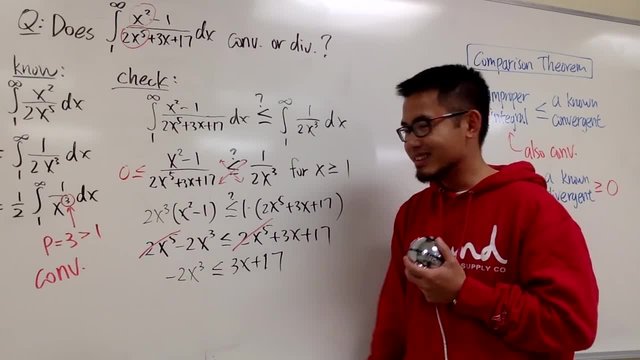 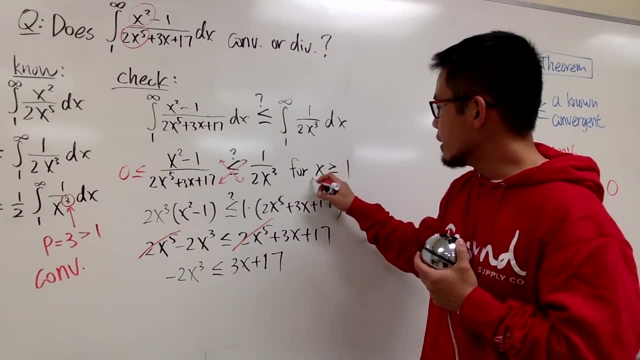 times 1 to the 3rd power is negative 1.. I mean negative 2.. And then plug in 2,, 3,, 4,, 5, so on. When x is greater than or equal to 1, this right here is always positive. 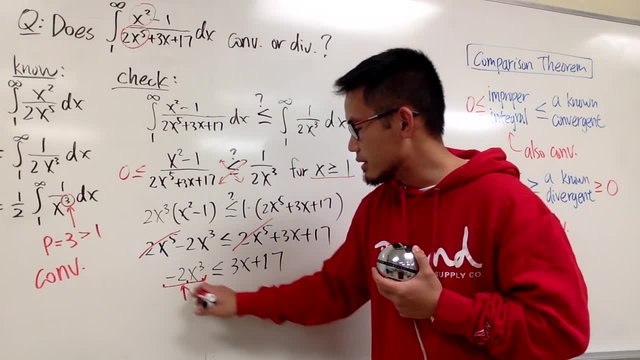 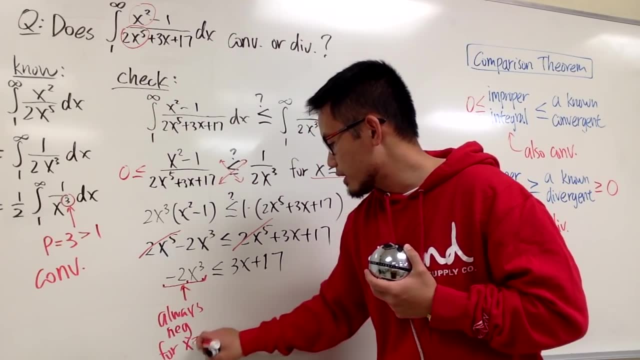 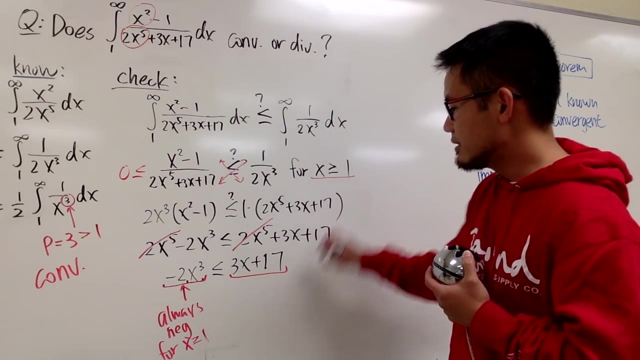 But then when you are multiplying by negative 2 together, this is always negative, for x is greater than or equal to 1.. All right, And on the right-hand side here, 3x plus 17,. this is always going to be positive. 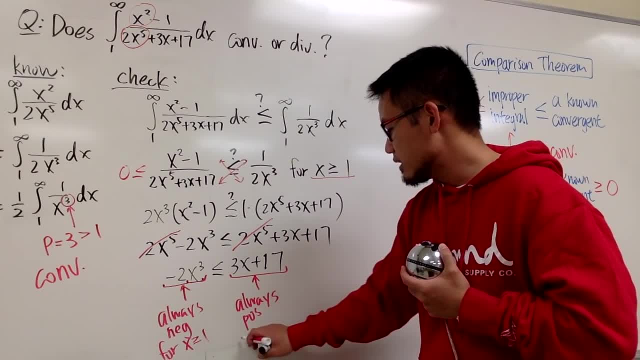 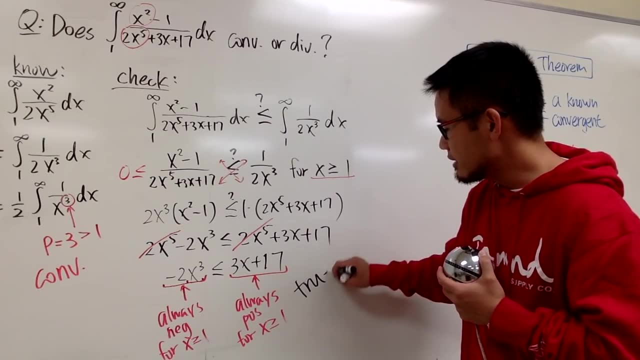 isn't it Always positive whenever you have x is greater than or equal to 1.. So, of course, right here I'm just indicating that this is true. Another way to show this is true is you can just provide me with the graph of this. 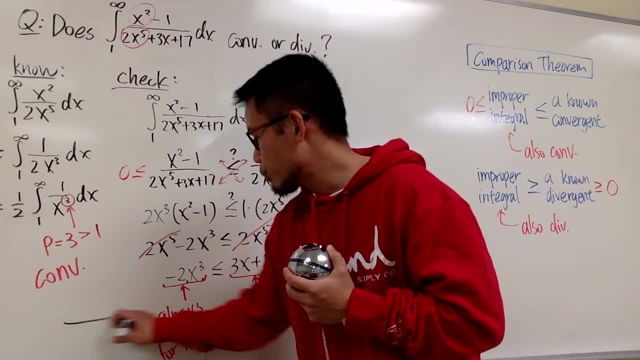 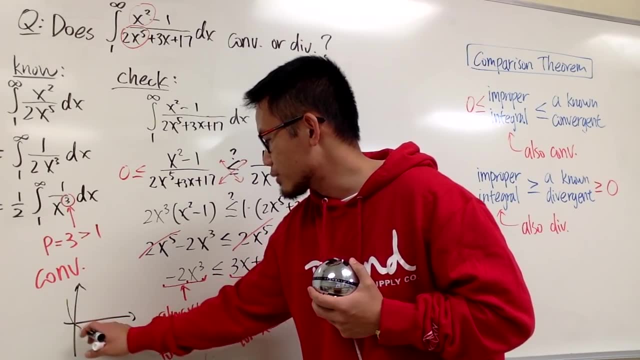 and the graph of that. So just real quick, if you want to provide a graph, the graph of this is going to be something down like this. right, I'm not going to draw a nice graph, something like that. It's always going to be down below here. 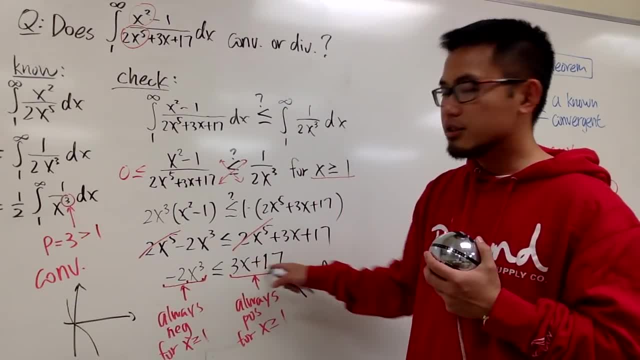 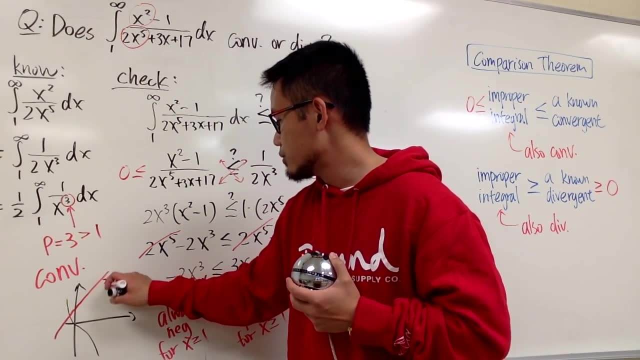 after you pass 0. And then this is just a line, right? So 3x plus 17 is going to be something like that. So this is 3x, This is 3x plus 17.. And this right here is supposed to be. 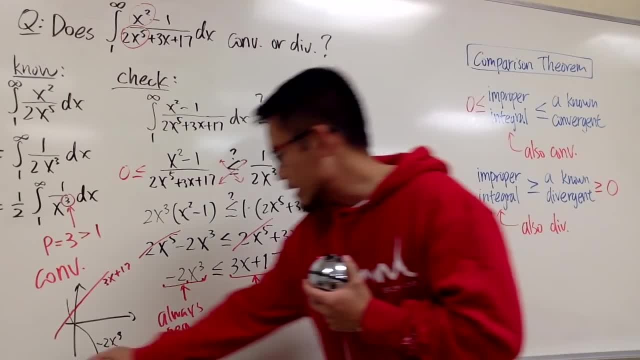 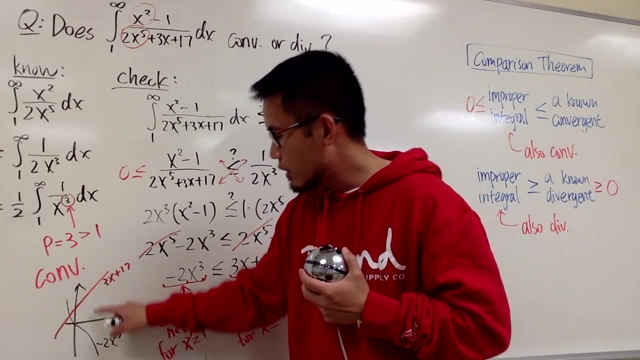 negative 2x to the third power. Okay, So you see that, because the graph of this line is always above the curve after you pass, x is greater than or equal to 1, right, So you know this is true, All right. 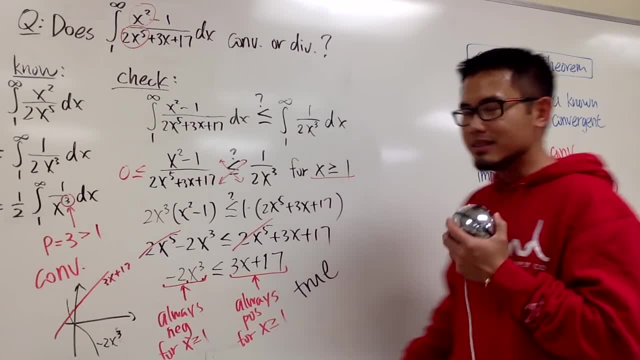 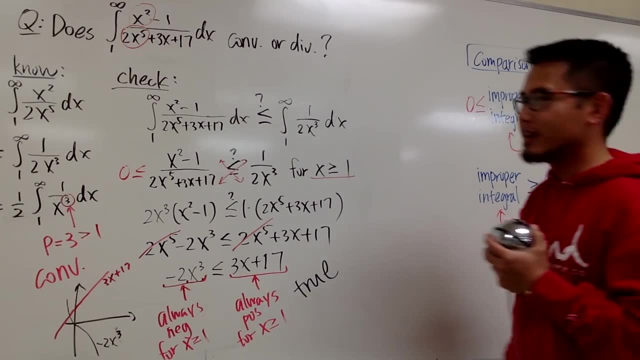 Now, because this is true, we have good news, because that will tell me we can draw a conclusion That can tell me that this improper integral that we're trying to find out this right here, also converges. So right here I just have to draw the final conclusion. 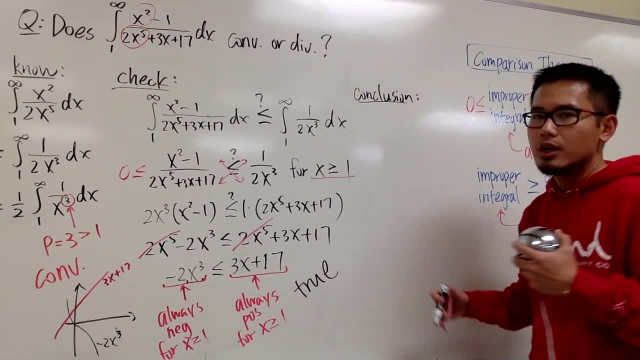 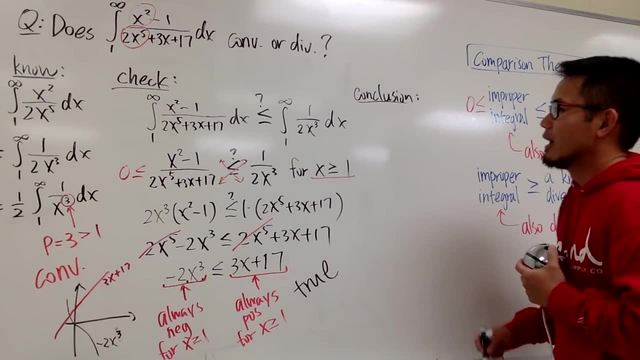 And seriously, this is just like how you will write your research paper or your English essay: Introduction party paragraph and then the conclusion, right. So here I want to just repeat the original integral again. I'll just write it down. 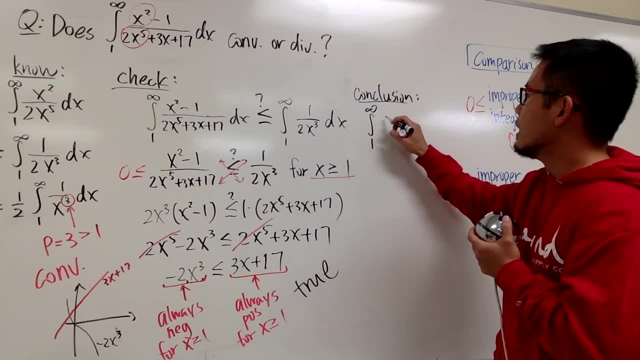 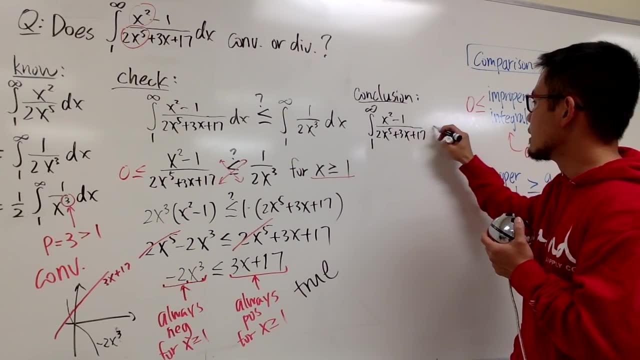 The integral that we're trying to do is 1 to infinity x squared minus 1 over 2x to the third power, 2 to the fifth power, plus 3x, plus 17 dx, of course, This right here Also.